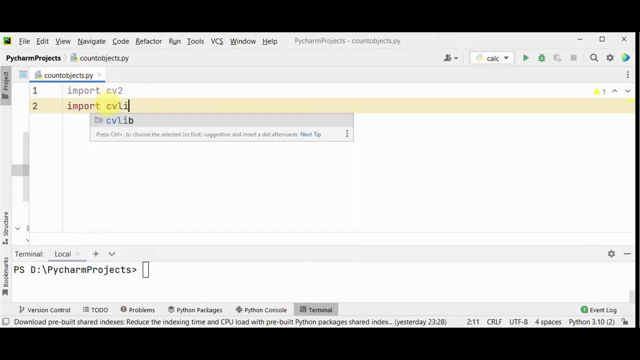 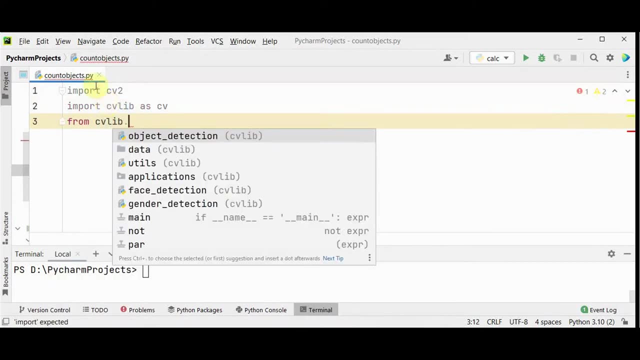 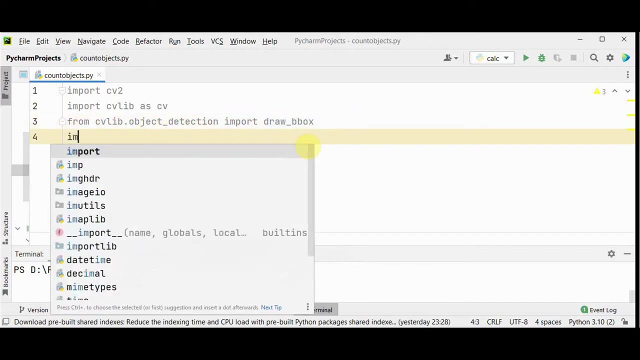 cv2, then import cvlib as cv. then from cvlib dot we need to detect the object first. so object detection, let's import and draw b box. this is to create a new image. and finally you can import matplotlib dot by plot to plot the image as plt. so initially we need to load the image for this. 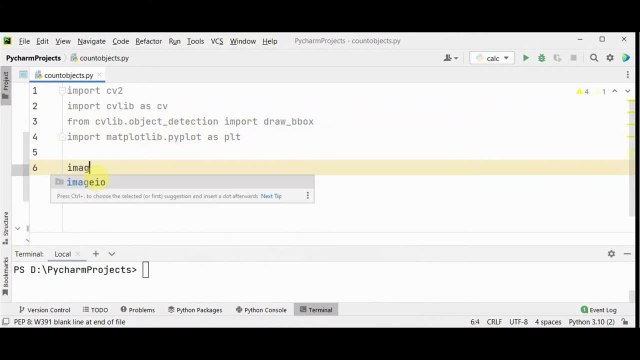 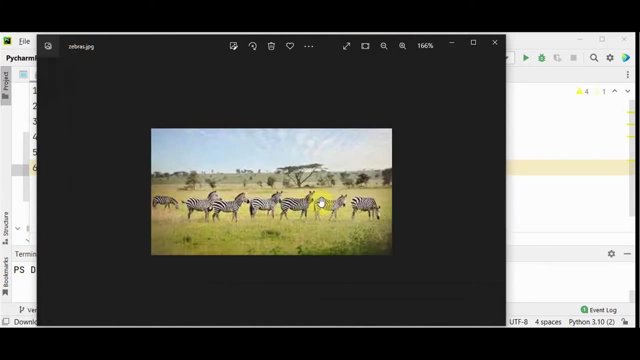 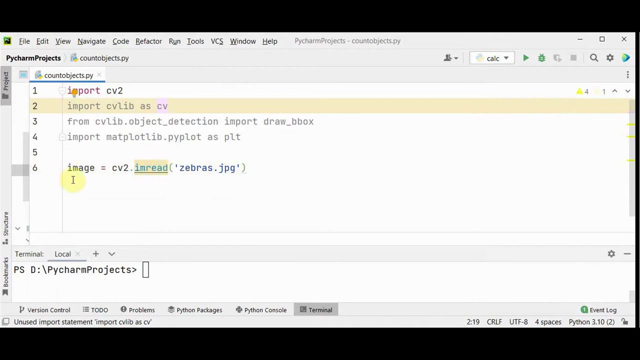 purpose. you can make use of imread method of cv2. store the output in a variable called image, equal to cv2 dot. imread method. pass the image as an argument here: zebras dot jpeg. so this zebrasjpeg file. this is present in the same folder as that of this python file. okay, so this method will return a numpy n dimensional array. 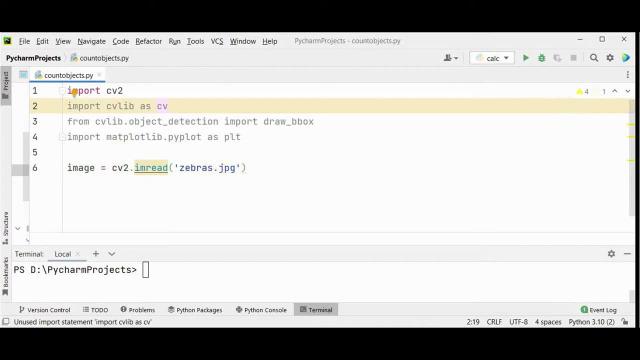 in case, if the image cannot be read, then it returns an empty matrix. after this we need to detect the common objects in the image. that is done through a function called detect common objects. so let me write the function first. cv dot- detect common objects. it takes this image, formatted as a numpy array, as the input pass image, and. 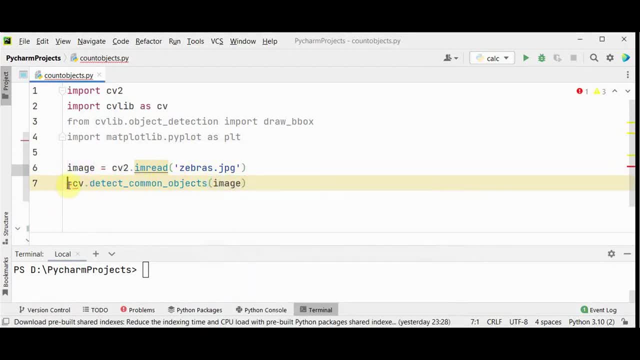 this will return three things. the first one is the list of bounding box coordinates, store it in a variable called box. and then list of labels for the detected objects corresponding to the index of the list of the bounding box coordinates. and finally, it will return a list of confidence score. 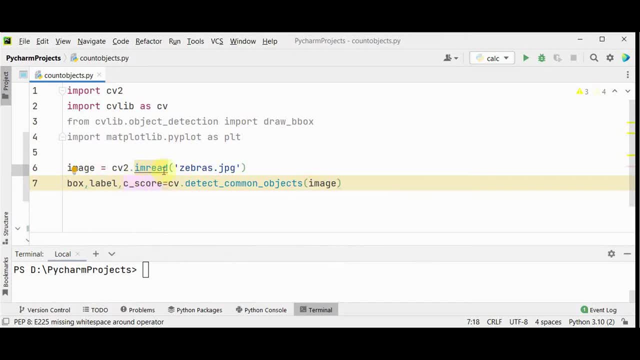 for the detected objects in the image. actually it shows how confident the model is that the predicted outcome is correct. okay, so the model used here is yolo v3 model, that is, you only look once model. so bounding boxes are just the rectangles that mark objects on an image. so in yolo format bounding box will be represented by four values: x, center, y. 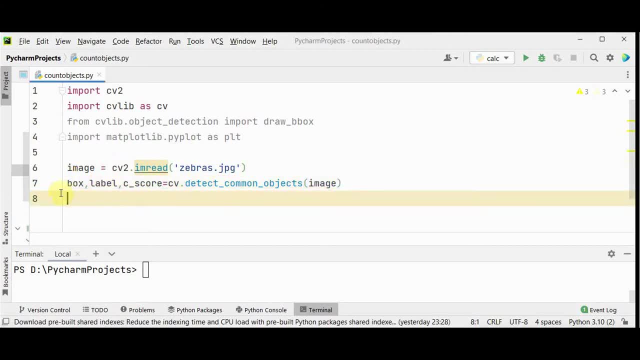 center, width and height. okay, then we need to create a new image that includes these bounding boxes. let me store the new image in a variable called output. to create a new image, you can use this draw bbox method. third, the first argument will be the image itself. then we have to pass these three values, that is.